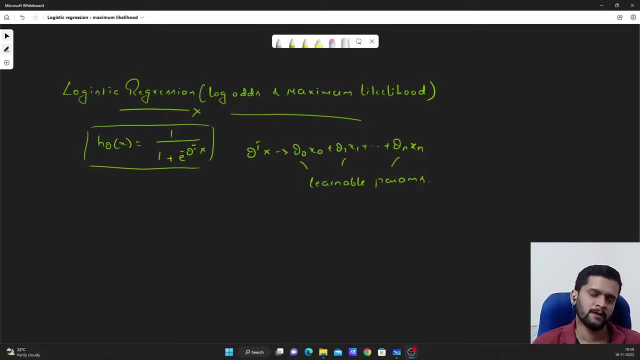 Hello guys, welcome to my YouTube channel. In this video, continuing our discussion on the logistic regression from the previous video where we have left, I will talk about log of odds and maximum likelihood, how a straight line is fit to the data set and that is in turn converted into. 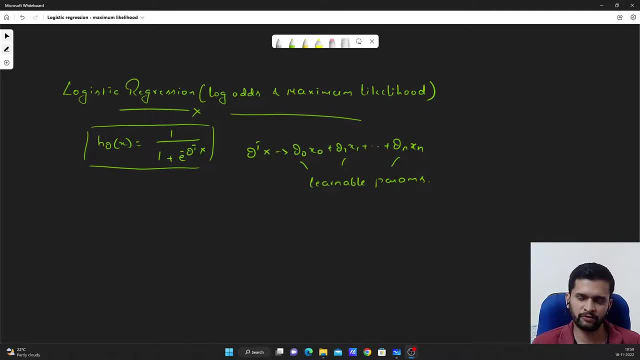 the sigmoid curve. So let us start. This video is going to be important in order to understand about log of odds and the probabilities, So please watch this video till the end. So, starting with, we have our hypothesis. So this is our logistic regression hypothesis. 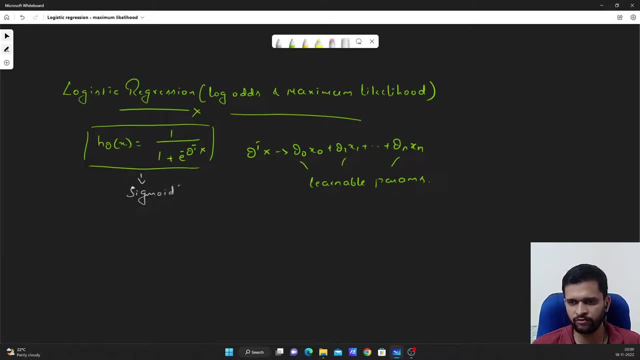 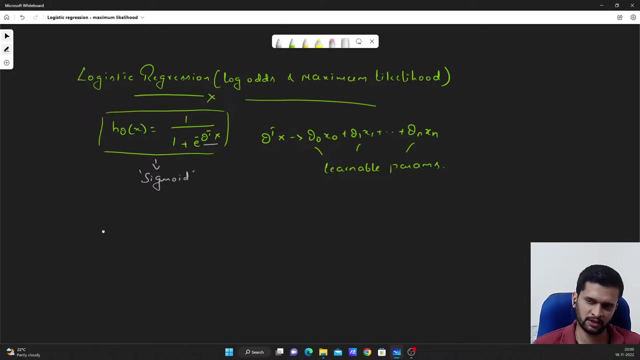 also called a sigmoid function. This is our sigmoid function, and this theta transpose x, in turn is represented as theta 0,, 8, 0, plus theta 1, x1, up to theta n, xn, and thetas are our learnable parameters. Now, in case of logistic regression, these thetas are presented in terms: 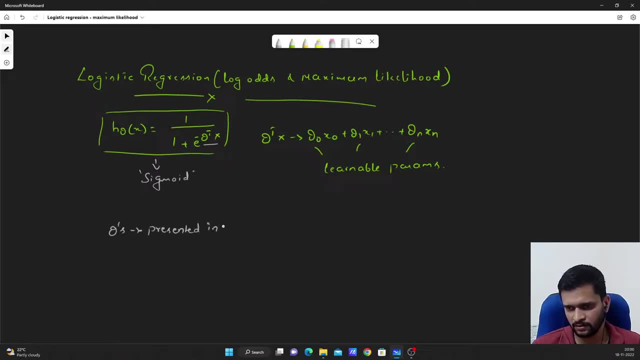 of log of odds and maximum likelihood, how a straight line is fit to the data set and that is presented in terms of log of odds. We are actually fitting a straight line initially to the given data points for classification and the parameters that we will be learning are presented in terms of. 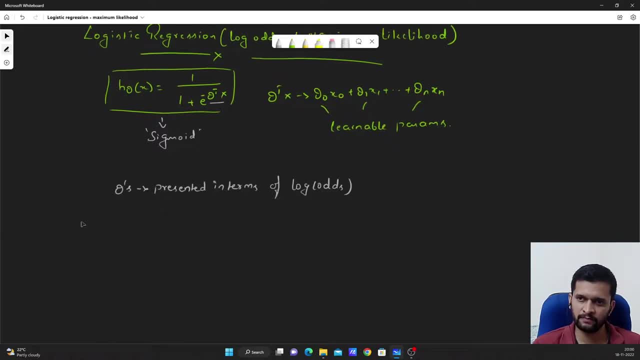 log of odds In order to fit the straight line. in case of linear regression, the y-axis would take the values from minus infinity to infinity. So in this case the y-axis would take minus infinity to plus infinity. correct, But in case of logistic regression, 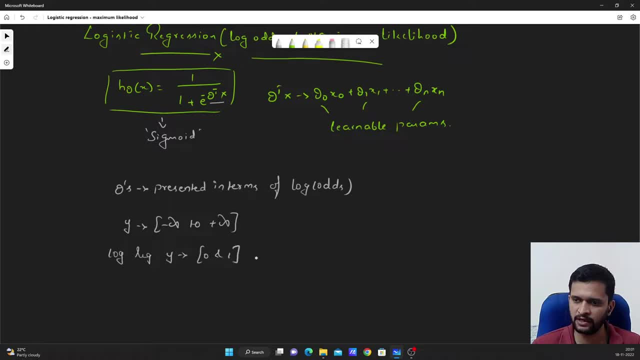 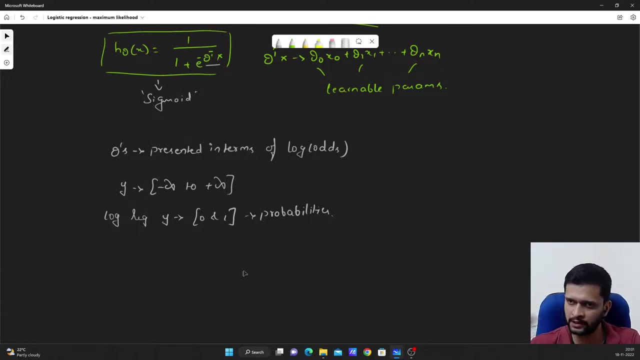 the y-axis takes only values between 0 and 1.. Why? Because these are our probabilities, correct Probabilities. So first we have to convert this 0 to 1 line on y-axis to negative infinity, to plus infinity, in order to fit a straight line. okay, So how we do that? So let us say: 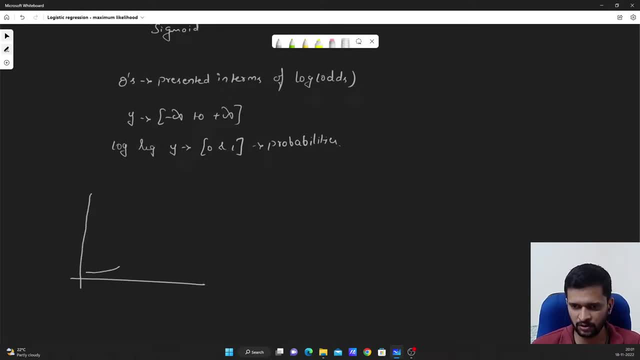 we have a sigmoid curve here. okay, It can be something like this: This is X, this is Y 0.501.. So this is our sigmoid curve. right Now, we will convert this to half the y-axis, values ranging from plus infinity to negative. infinity. So this X reach to minus infinity, then x is 0 and 1.. So we have to cover the last part of our점 And we are using zero, which is zero at the top, And then we will. provide this value as minus infinity 0.. пр po figure infinity- Cas and r nochmal everything right. So that is just a cherry on the other side него. So let us convert this x, the y-axis, and minus infinity to negative infinity, to plus infinity, to positive infinity. 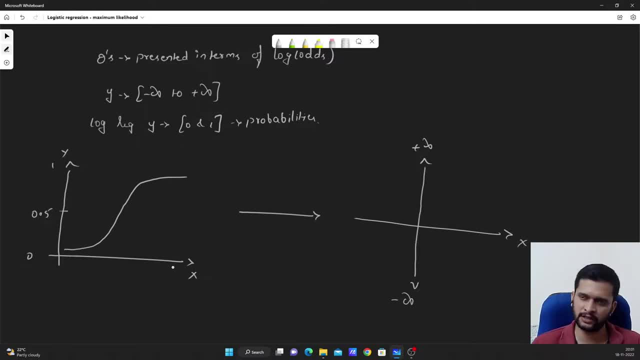 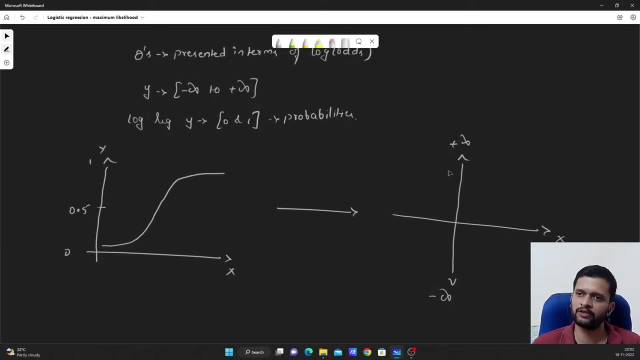 um состав. So this is the pediatric information For this. so let us NOT convert it. x remains same as of this axis. ok, Now how do we convert this y axis from 0 to 1, to negative infinity, to positive infinity? So, in order to convert this, we make use of log of odds. 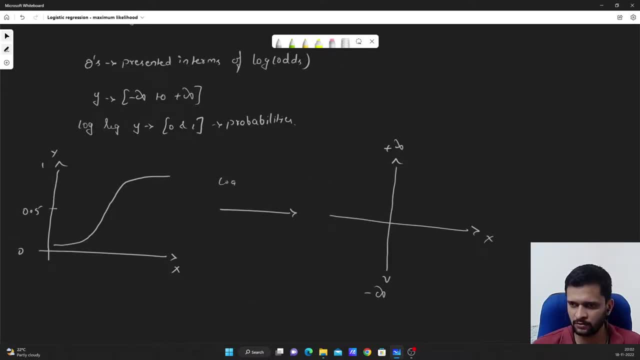 ok, So there is something called as log of odds, and the formula for that is log of p by 1 minus p. ok, So this will be 0,, 1, 2, 3, up to so on, so on, up to positive infinity. 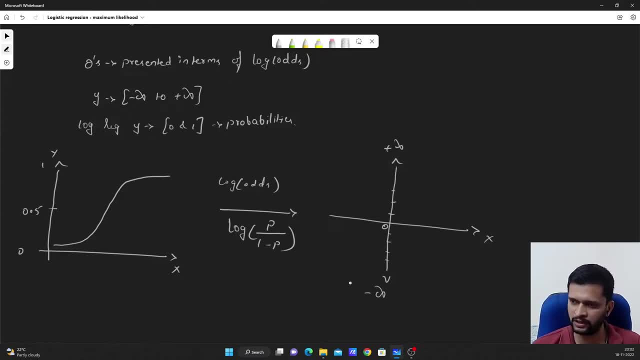 like this: minus 1, minus 2, minus 3, so on up to negative infinity. So this 0.5 to 1 will be converted. it to 0 to positive infinity. 0.5 to 1 probability will be converted into. 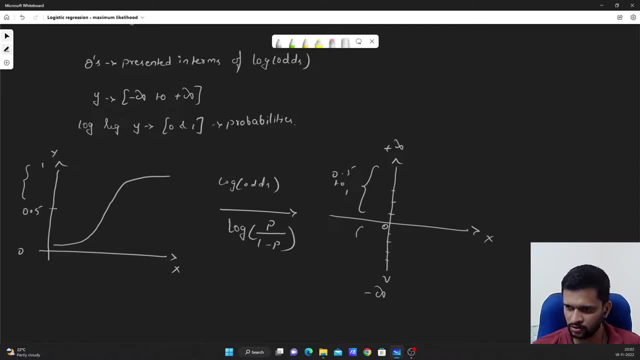 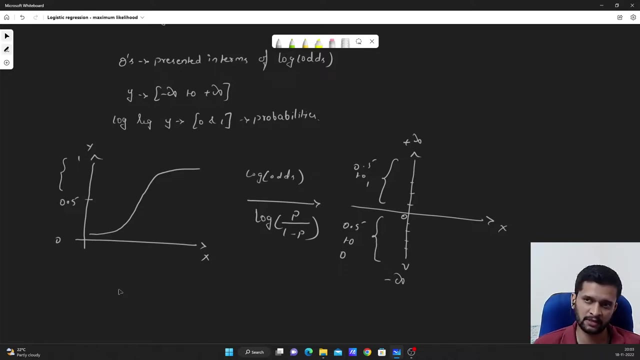 0 to positive infinity log of odds- right, So, similarly, from 0 to positive infinity log of odds. ok. From 0.5 to 0, the log of odds would range from 0 to negative infinity- ok. So this is how we convert our sigmoid, or the probabilities on y axis, which are ranging from 0 to 1. we 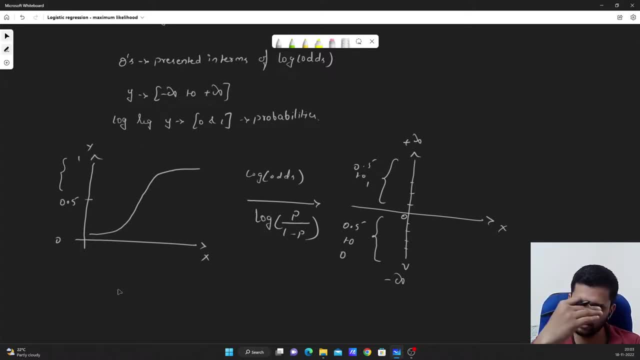 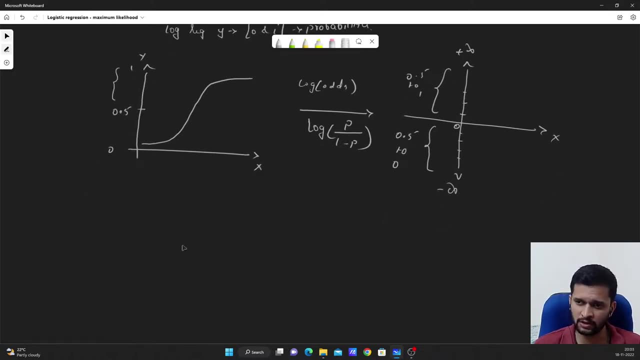 convert them to log of odds, which will range from negative infinity to positive infinity. ok, Now, now that we have converted the probabilities to log of odds, what we do? What we do is we fit the candidate line to the data points. ok, So this is our x axis, this is our y axis. 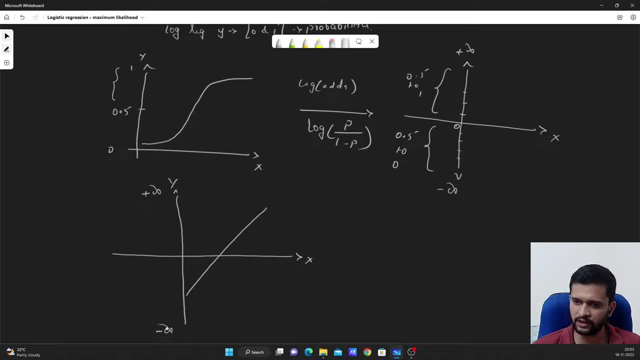 this is positive infinity. this is negative infinity. right Now, let us say we have the data points at negative infinity, whose probabilities are 0. ok, So the probabilities are 0 would be situated at negative infinity. whose probabilities are 1 would be situated at positive infinities. 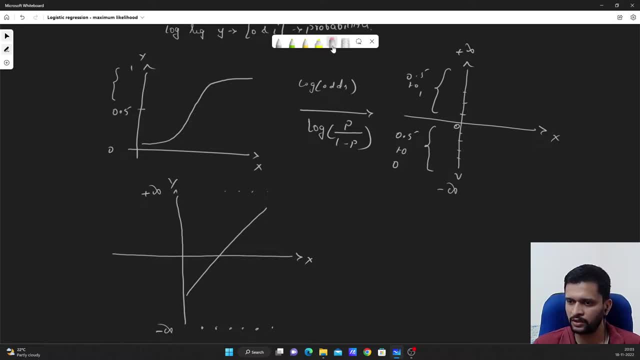 ok, So we can do something like this, right? So let me just redraw it so that you would not be confused. So it will be looking something like these things: ok, Now we will consider this as our best fit candidate line. best fit candidate line, If you can relate it to. 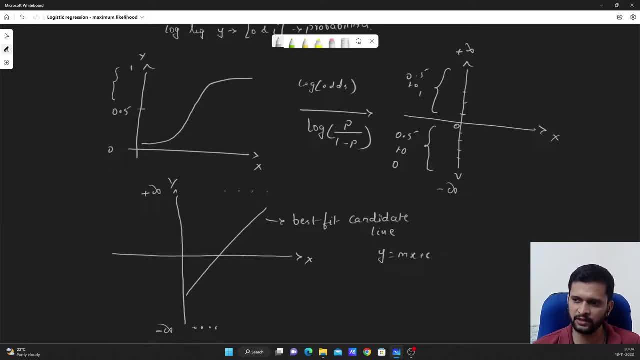 the equation of straight line, y is equal to m, x. So m is a slope of the line. So for each unit increase in x, by how much y will be increasing or decreasing? that will be determined by value m right. So in case of univariate, 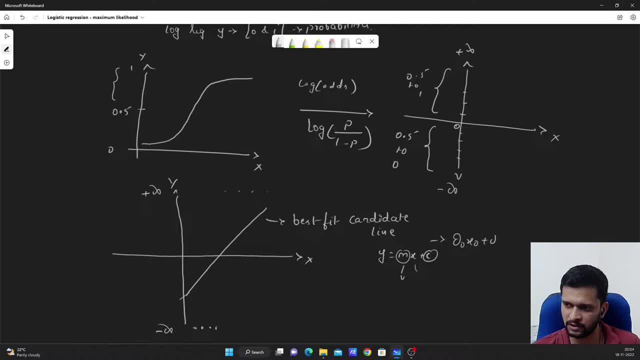 linear regression. if you consider the simple example: theta 0- x0 plus theta 1- x1- right. So this relates to x. here this m will be theta 1 and c will be theta 0, right. So this is the slope of the line now. So this is the slope of the line and this is the slope. 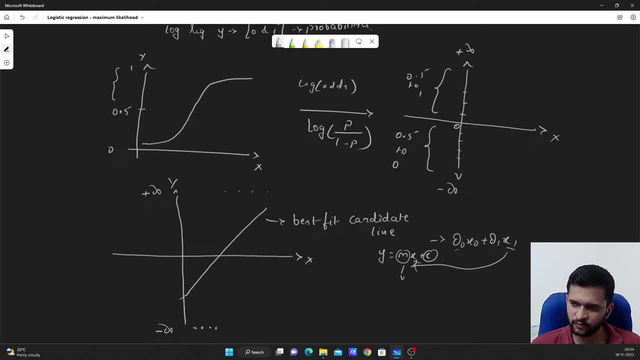 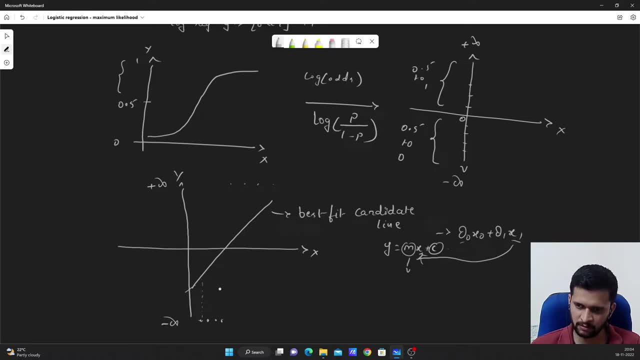 of the line y and this is the slope of the line. Now this beta 0- x0 plus theta 1 minus delta 1- x1, right So should be taken as the upper limit of the string, which is x equal to right. so now what we do is we will project these data points on this best candidate line that we 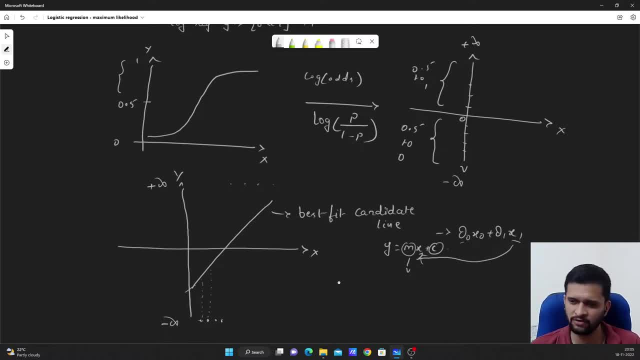 have initialized. okay, based on the initialization of theta values, we arrive at this particular line and we project our actual data points onto this particular line. right? so these are our projections. so this point will be projected over here. this will be here. this will be projected over here. 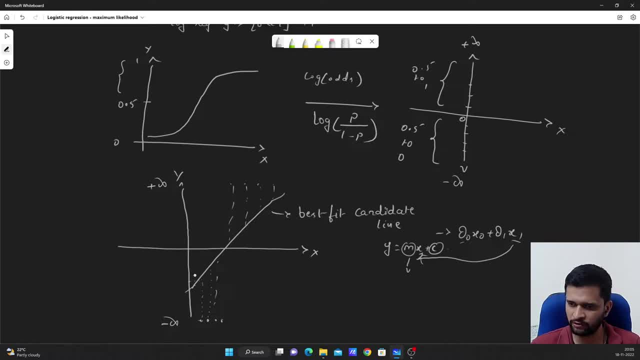 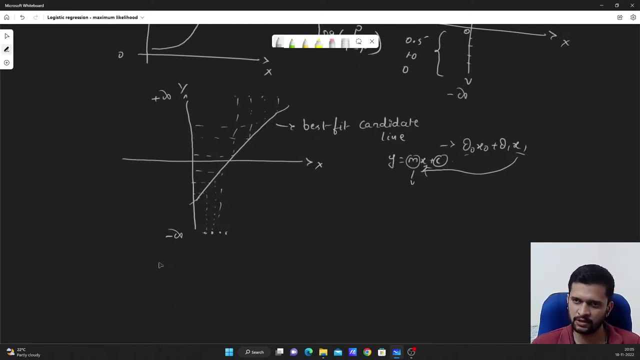 now, for each of these data points, the corresponding value on the y-axis is the log of odds. okay, so log of odds, correct. now, now that we have log of odds for each of the data points, we will convert these log of odds back to probability so that, instead of 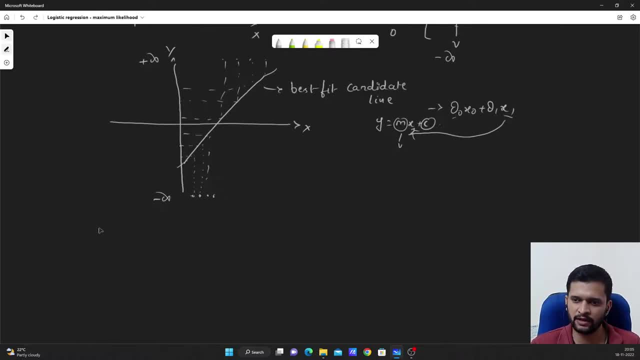 this particular straight line, we can again get back to our sigmoid curve, right. so how we can get back to our sigmoid curve, right, so how we can get back to our sigmoid curve, right, so how we can do that. so all we have to do is we have to substitute in this particular formula: 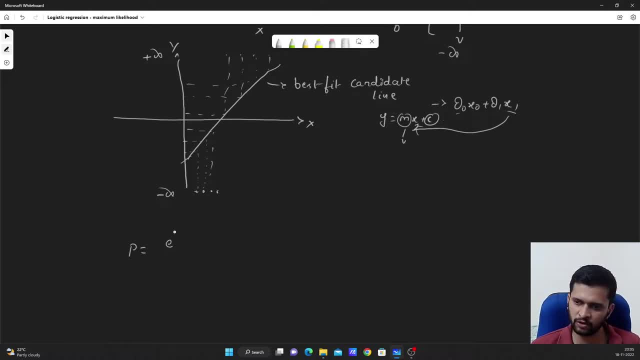 probability using log of odds is calculated as: p is equal to e power log of odds divided by 1, plus e to the power log of odds. okay, so this is how we convert the log of odds into probability. again, once we convert the log of odds into probability, the values will be between 0 and 1. 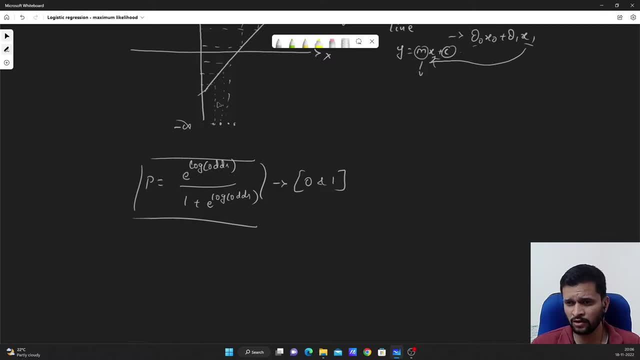 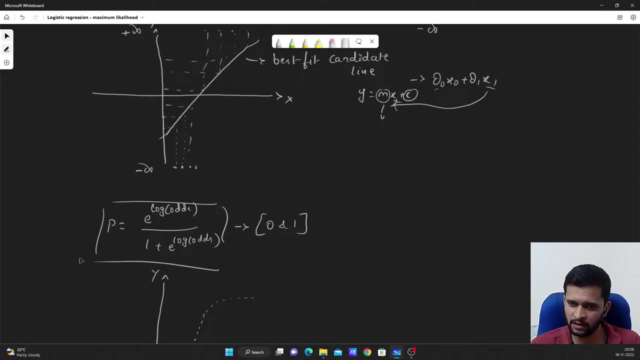 right now, based on the log of odd values for each of the data points that we have, we will convert it into probability and plot it according to the probability that we get x and y. so this particular line now is shrunk and turned into the shape of this s curve, the sigmoid curve. okay, 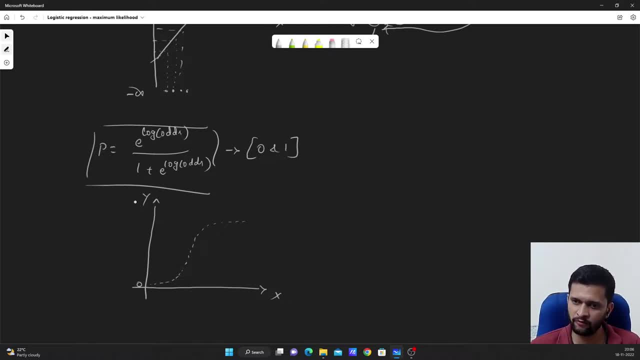 And the range of values it can get is 0 and 1, why? Because we have calculated the probabilities from log of odds that we have arrived at in, arrived in the previous step, in this particular step. ok, Now that we have these probabilities right, so these probabilities are also called as: 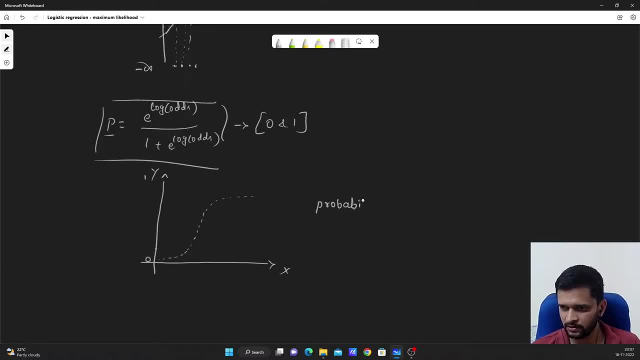 these probabilities are also called as the likelihoods of the individual data points. Why these are called as likelihoods? Because we have calculated these probabilities based on the log of odds. right, We are not considering this probability as area under the curve, ok. 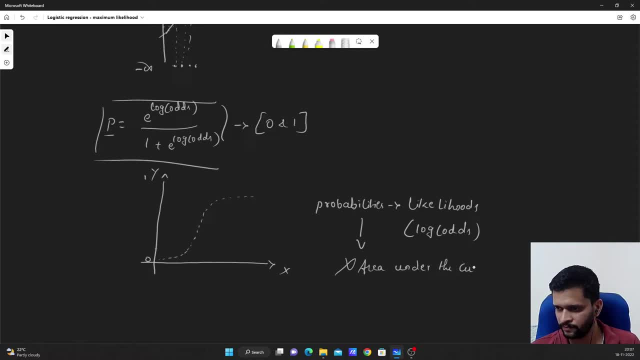 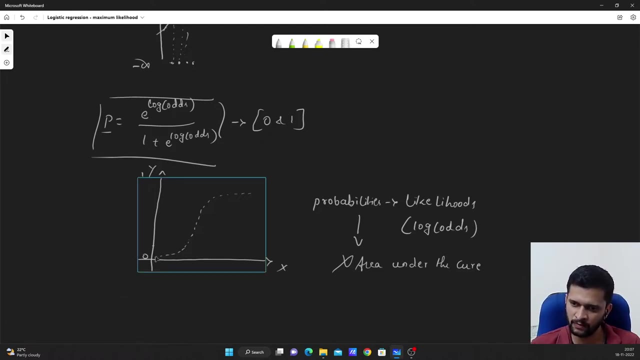 Just remember this. this is not area under the curve, Anyway. Instead, this is a likelihood. why? Because we have calculated the probabilities using log of odds. ok, So now we have converted log of odds to probabilities and then we have arrived at this particular 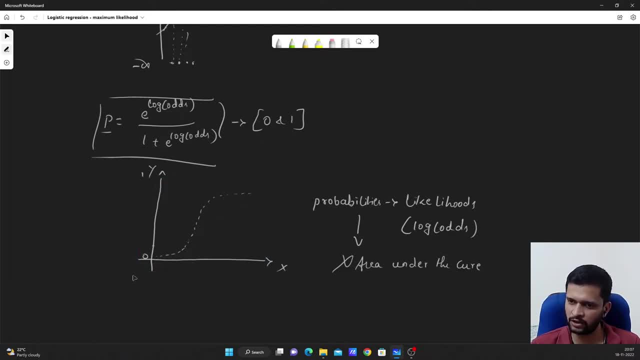 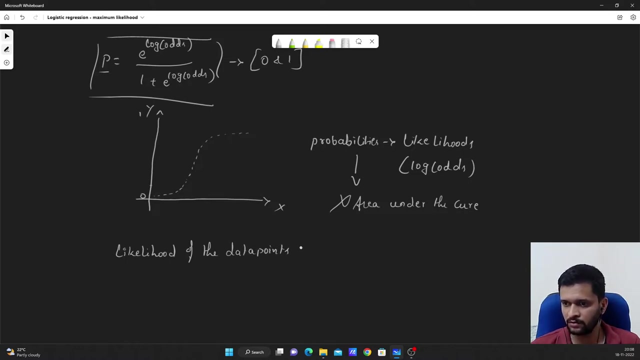 sigmoid curve: ok, This is our sigmoid curve. We have shrunk the straight line into this particular sigmoid curve. Now that we have arrived at this particular curve, we calculate the likelihood of likelihood of the data points given this sigmoid curve. ok, 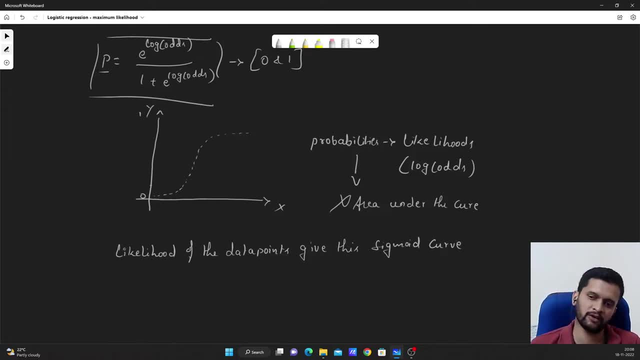 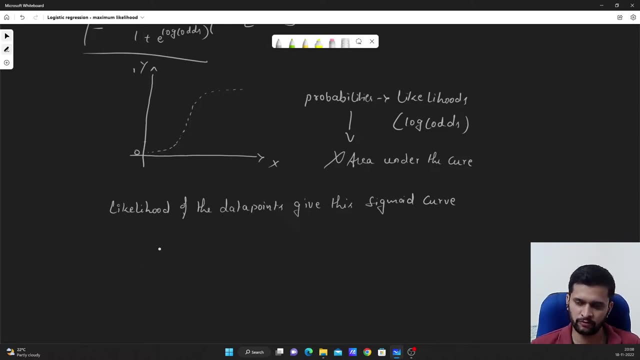 Based on the sigmoid curve, we calculate the likelihood of the given data points. So how do we calculate the likelihood of the data points? So for that, let us consider: we have only three examples, ok: X1, X2, X3, ok. 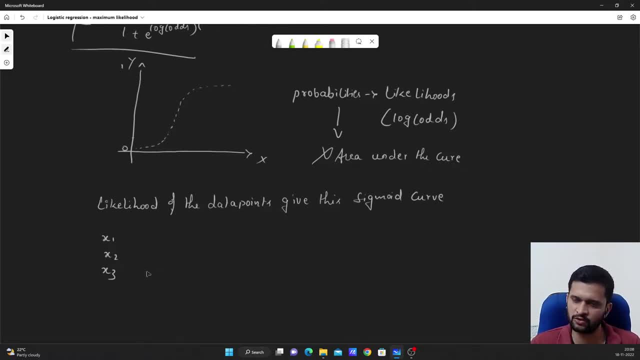 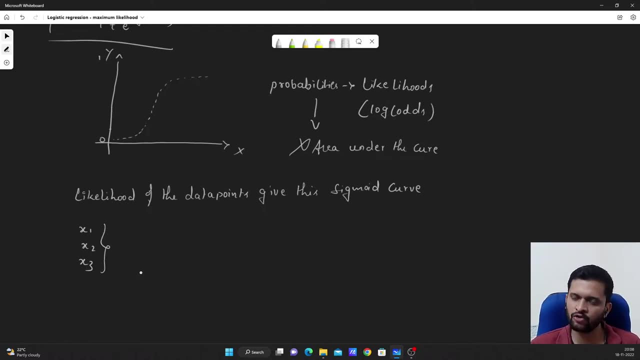 And this is a univariate regression problem. It has only one independent variable and one independent variable. Now that we have these three examples, how do we calculate the likelihood? So, in order to calculate the likelihood, all we do is we multiply the probabilities. 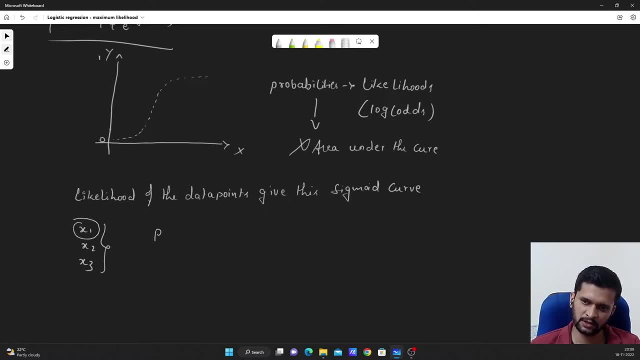 of this particular instance belonging to class positive with with the probability of this particular instance belonging to class negative. similarly, we multiply all the probabilities for all the instances. so how can we write that probability that x 1 is equal to 1 into probability that x 2 is equal to 1, into probability that x 3 belongs to class 1? 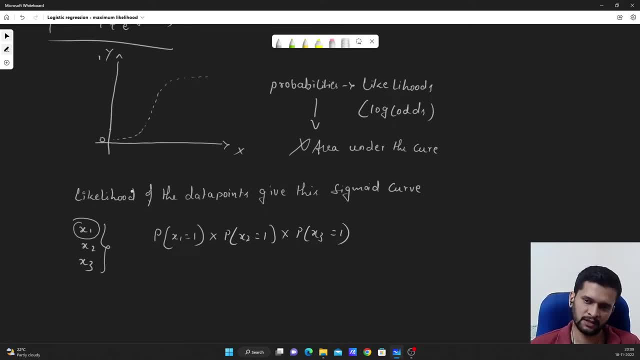 so, for example, you can consider: these three are our size of the tumors. okay, size of tumors. and this probability equal to 1 means the probability that these data points belongs to cancerous, cancerous category. okay, so this is probability that these three points belong to cancerous category. similarly, we multiply with these three data points belonging to: 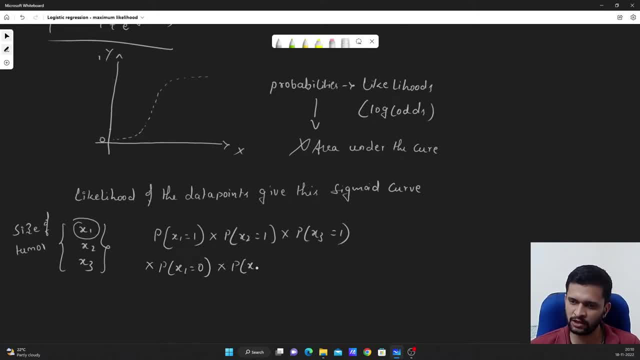 non-cancerous category. so this is probability that x 2 is equal to 1. into probability that x 3 belongs to cancerous category. so how we can mention that x 1 equal to 0, probability that x 2 equal to 0. into. 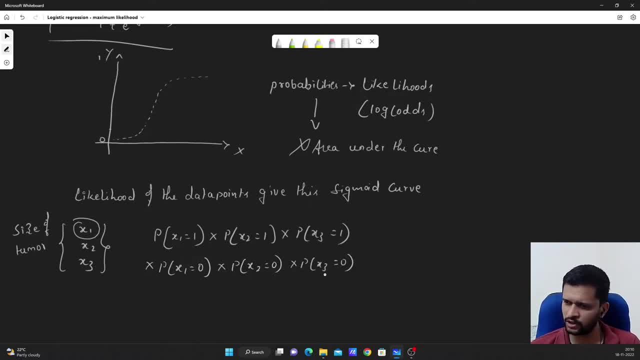 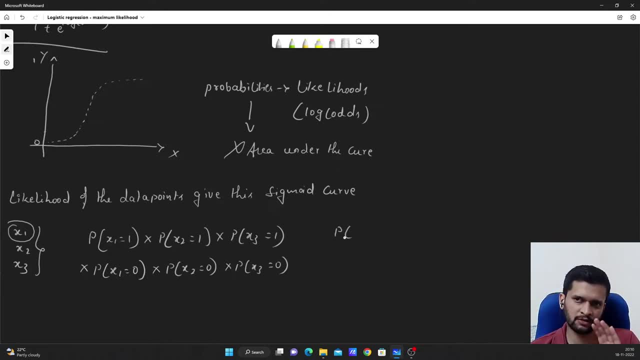 probability that x 3 is equal to 0, right? just remember. the probability will always equate, always range from 0 and 1, right? maximum value can have is 1. so the probability that a given data point belongs to 1, plus probability that a given data points belongs to class 0, always. 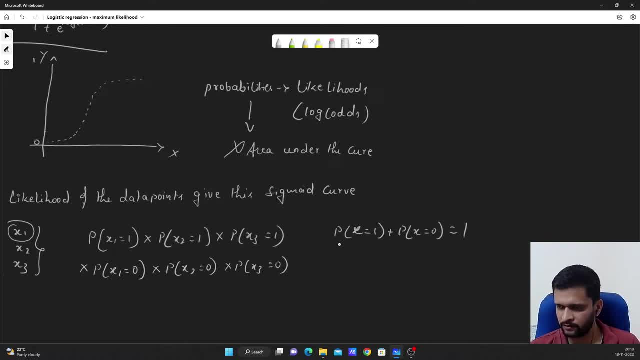 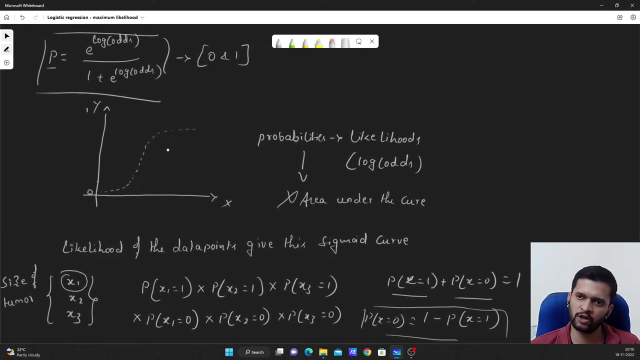 equates to 1, right? so since we have probability that x is equal to 1, how we can calculate probability that x equal to 0? it's simple, right. it's 1 minus probability of x is equal to 1. this will give us probability of x equal to 0, correct? now this line gives us the probability that each data point. 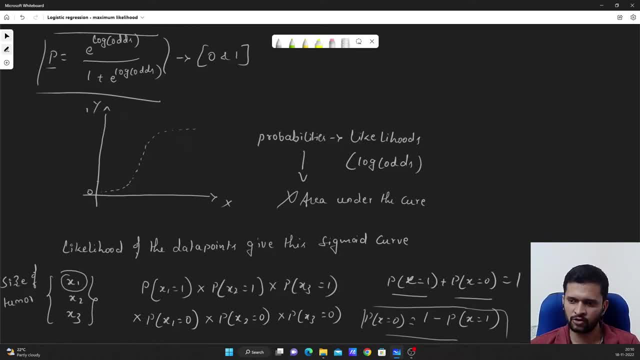 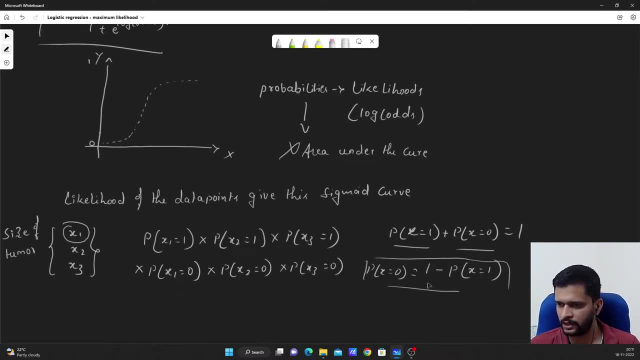 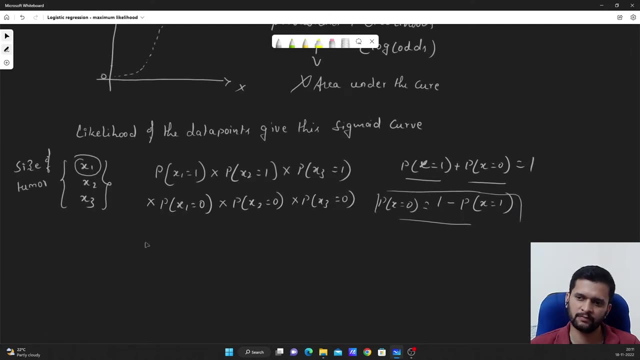 belongs to positive class. okay, so we can calculate the probability that x is equal to 1. right, so we can calculate the probability that each data point belongs to negative class. how, using this particular formula and calculating this likelihood? now, instead of multiplying the values, to make it easy, we apply logarithm to this product. okay, after applying the logarithm? 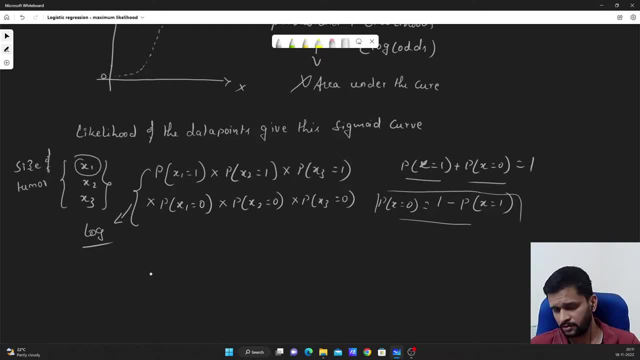 this multiplication will get converted into addition. okay, so that's the property of logarithm. so after this the equation becomes log of: x 1 is equal to 1 and x 2 is equal to 1, right? so I will just write p is equal to 1 into log of. I will just say p 1 equal to 1 and. 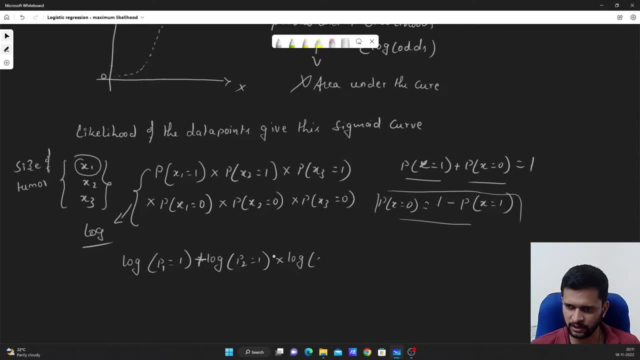 p 2 equal to 1 into log of. okay, sorry, this is not multiplication. now this will be plus, because we are applying logarithm: log of p 3 equal to 1, plus log of p 1 equal to 0, plus log of p 2 equal to 0, plus log of p 3 equal to 0. 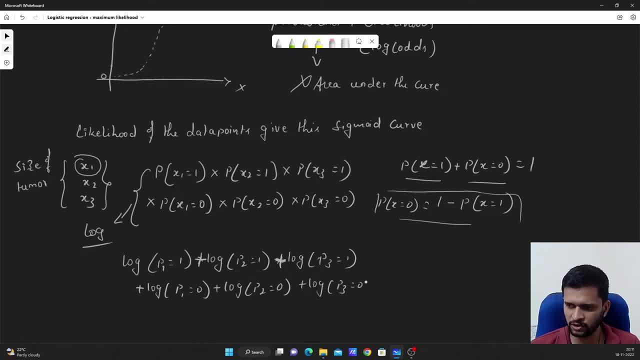 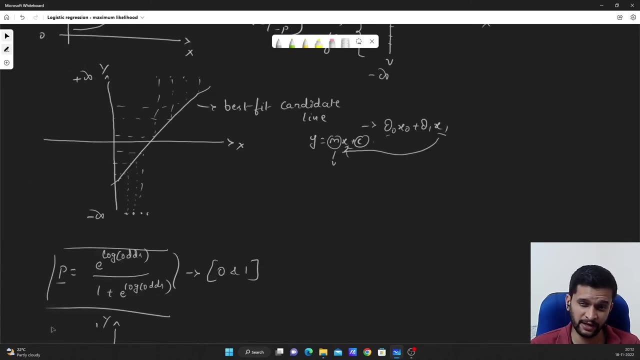 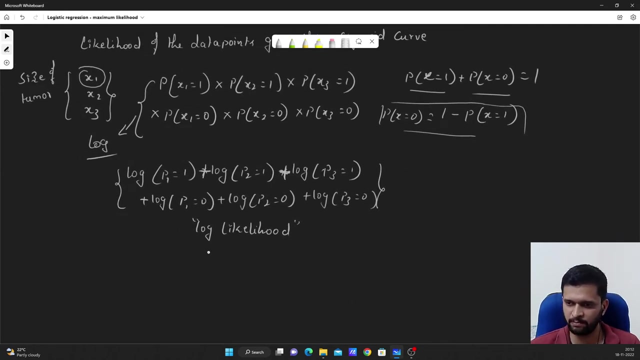 So after this we can get a gradient here now where we want to find the loss of tau in equal to 0, right. So this is our log of likelihood right Now for any candidate line that we had earlier initiated. we want this log of likelihood to be maximum, okay. 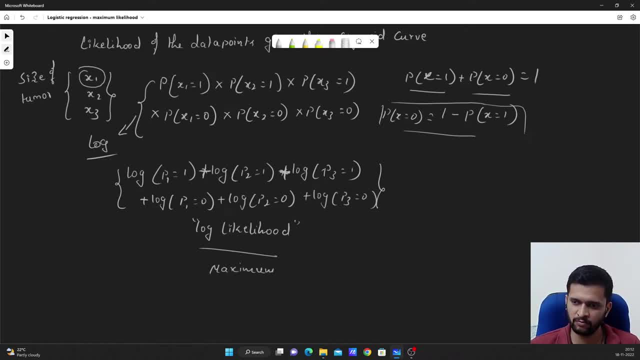 We want this to be maximum value. Why we want this to be maximum? Just think and answer it in comment section. I will provide the answer in the description after few days, once you guys have come to the answer. okay, If you guys do not understand how it works, just 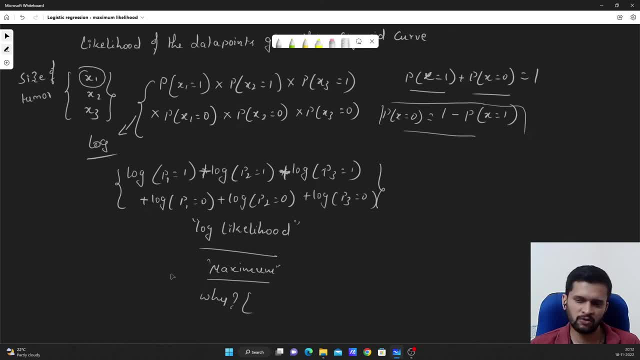 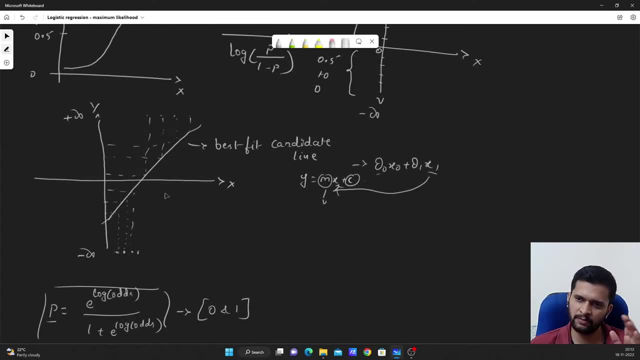 post in comment section. I will get back to you Now that we know we need this value to be maximum. in the next iteration, this particular line will be rotated. Let us say it takes this particular orientation. Now, based on this orientation, the log of odds will change for each of the data points. 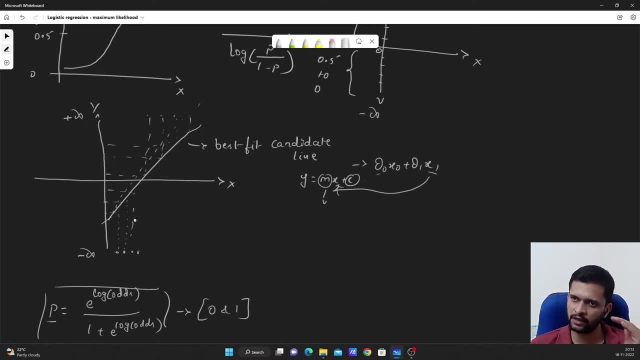 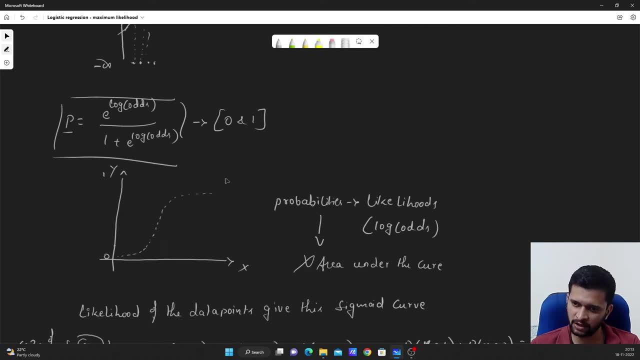 Since the log of odds changes, the probability or the likelihood changes for each data point. Since the probability changes the likelihood of this particular shaped curve, this shape will also get changed. As the orientation of the line changes, the shape of this particular sigmoid may also. 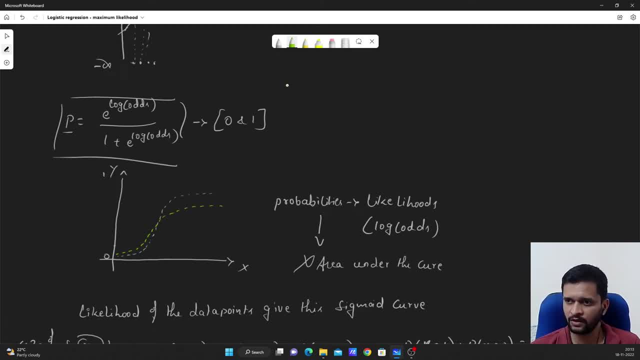 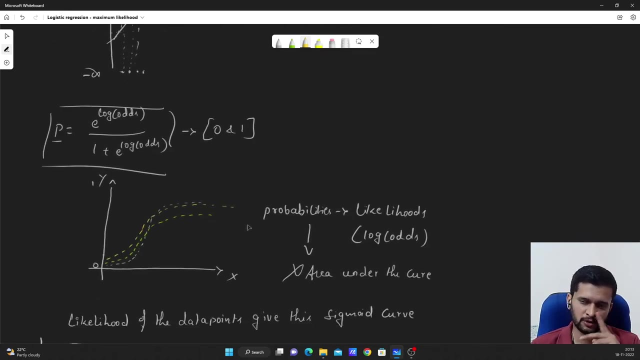 get changed. So this may look like this, or it may even take the form somewhere like this. So it depends on the orientation of the line. the shape of the sigmoid curve will matter. So once we have this, we calculate the log of all, the log like log, likelihood of all. 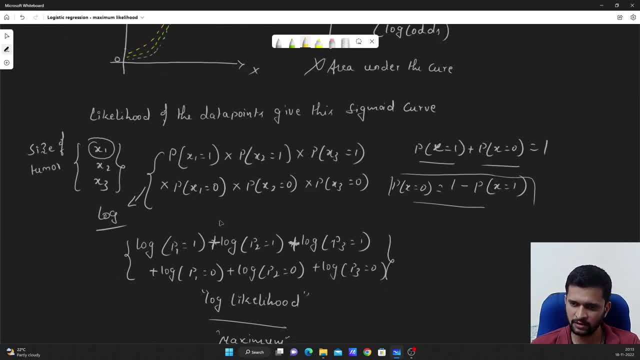 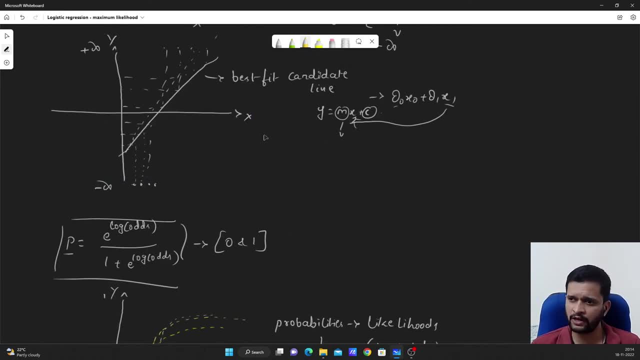 the data points. So that means we have this particular line. So let us say that we are data points using this particular formula here and we want this to be maximum. so for the different orientation of this particular line, we will have different parameters, right, thetas. so based on the 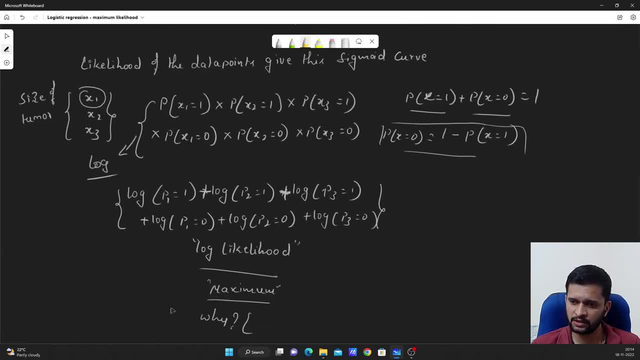 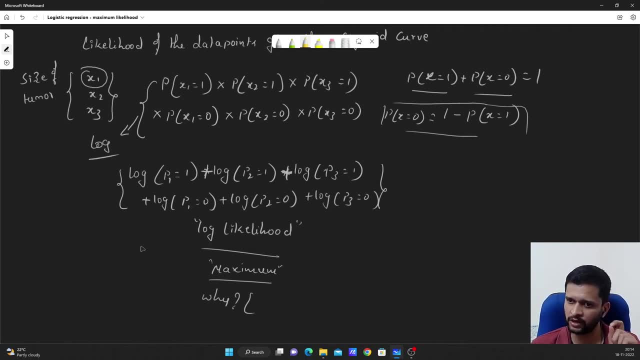 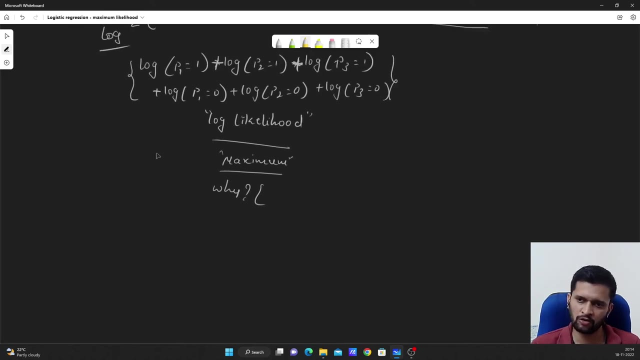 parameters, thetas, which give us this maximum value for the log likelihood, we will choose those particular parameters. okay, so this is all about maximum log likelihood. now, if you can relate this log likelihood or log of odds- sorry, not log of odds- just relate this log of likelihood to the 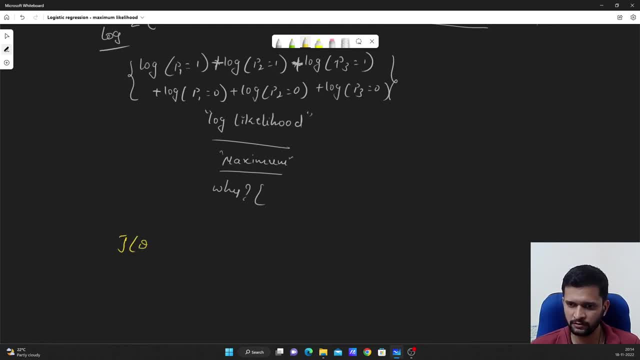 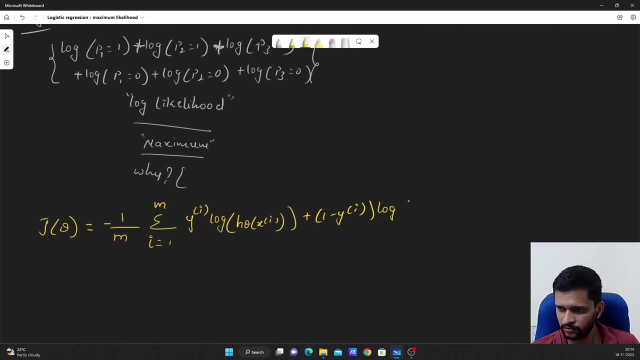 cost function that we have. j of theta is equal to minus 1 by m. summation of i is equal to 1 to m. right y i into log of h theta of x i correct and then 1 minus y i. I will just move this aside. 1 minus y i into log of 1 minus s theta of 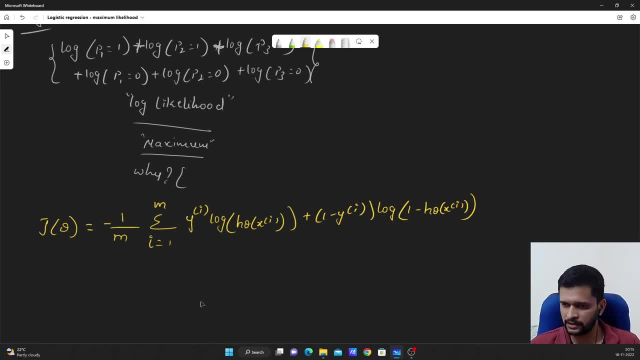 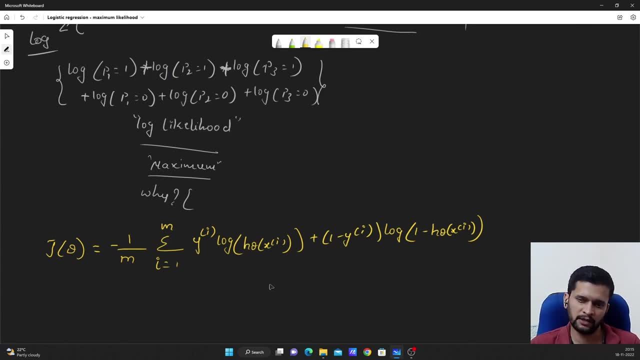 x, i. So if you guys can see any resemblance between the maximum likelihood calculation formula and the cost function formula, I think you guys would understand why we say maximum likelihood here and why we have to minimize this cost here. We have to minimize this cost.